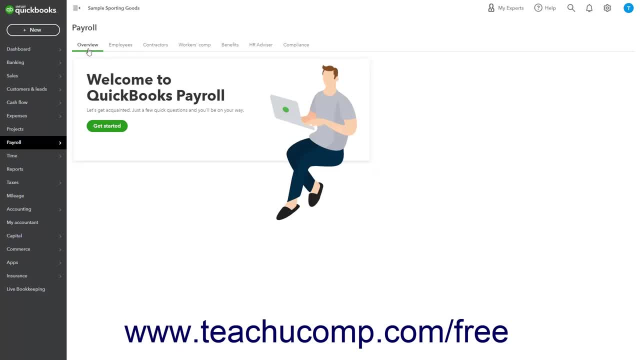 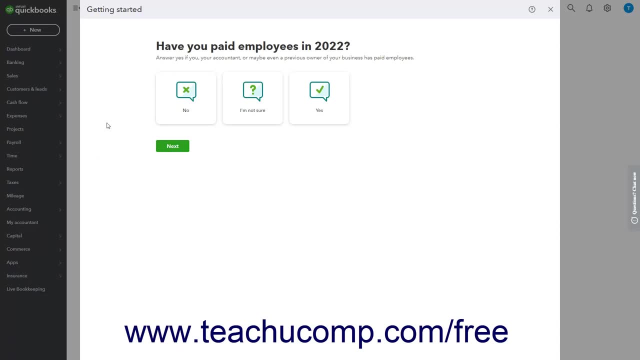 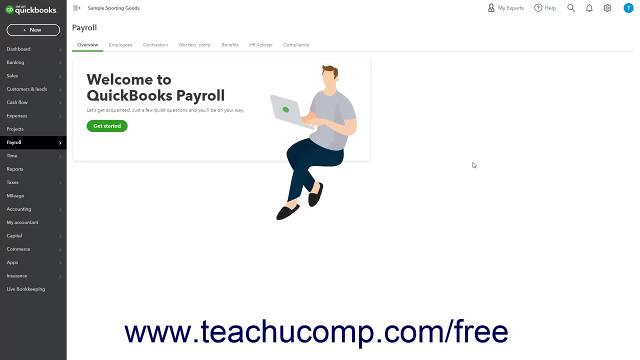 You'll then be redirected to the Overview page of the payroll pages, where you can then click the Get Started button to set up payroll before adding your employees. You can also add employees as part of the initial payroll setup, if desired. Alternatively, to add employees for time tracking. 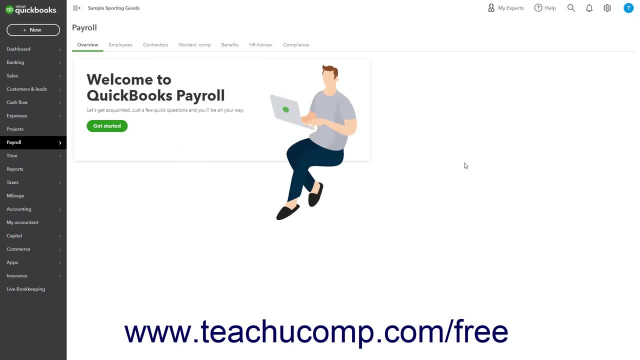 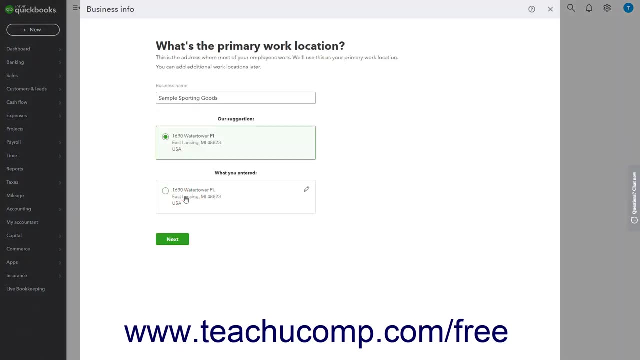 with a pay kit. click the Add Employees tab at the top of the page. Thus your employees will be a payroll plan. click the Add an Employee link instead and enter the employee's information to record in the Employee pane that opens To create a new employee and or invite the employee to enter their payroll information. 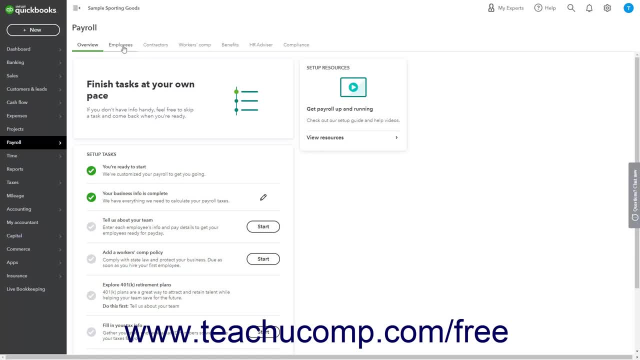 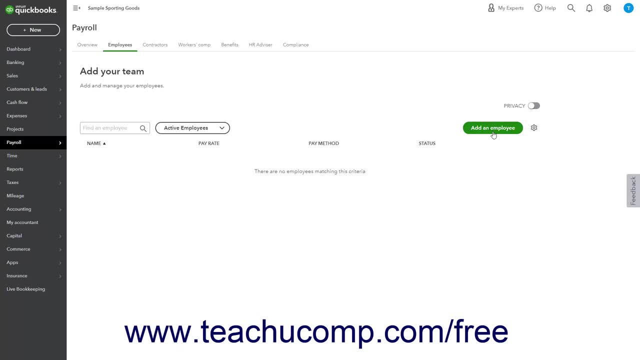 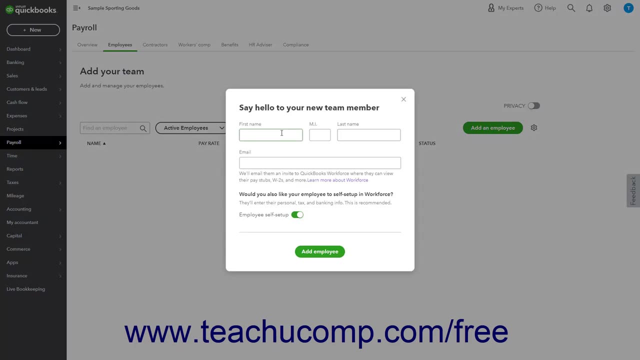 into QuickBooks Workforce. after setting up payroll, return to the Employees page and then click the Add an Employee button in the upper right corner of the Employees list to open a Say Hello to Your New Team Member window. First enter their name into the First Name, Middle Initial and Last Name fields. 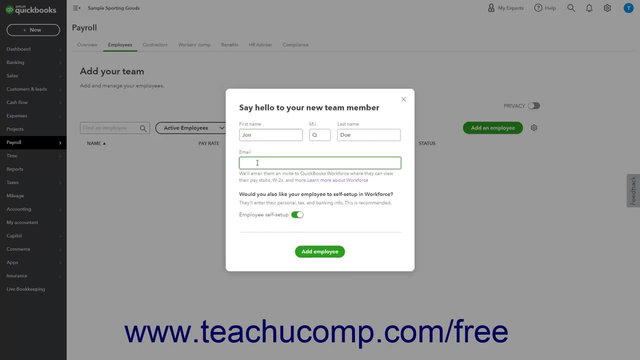 Then enter their email address into the Email field To then let the employee enter their own personal tax and banking information. ensure the Employee Self-Setup toggle switch is set to the On position. Alternatively to manually enter this data for them, click the switch to toggle it off. 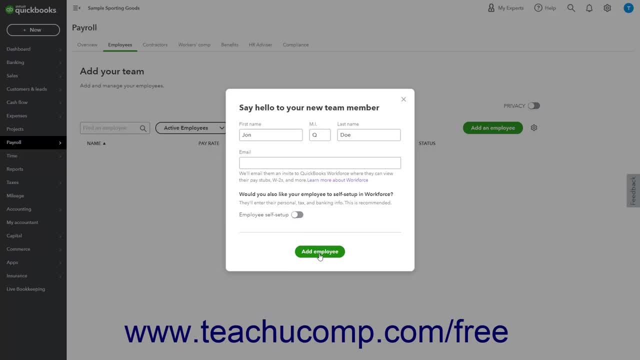 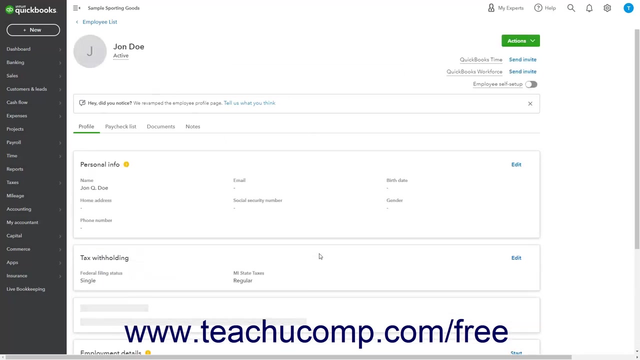 Then click the Add Employee button to send the invitation and or create the employee. If the employee is sent an invitation, then they can log in and enter their payroll information After creating the employee. you can then see the employee's details within the different 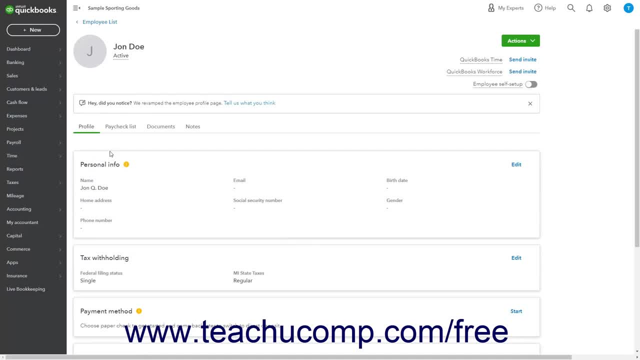 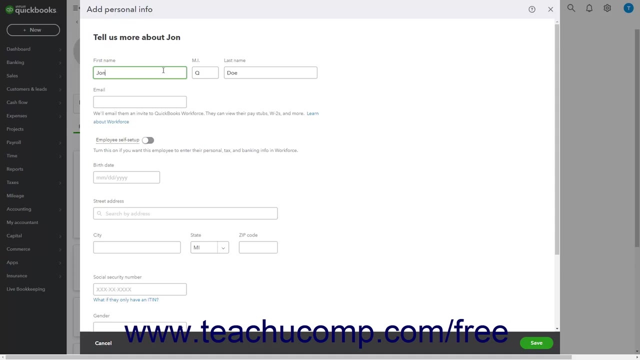 sections that appear on the Employee's Profile page. on the Profile tab To edit their personal information. click the Edit link in the upper right corner of the Personal Info section to open an Add Personal Info window. The employee's name appears in the First Name, Middle Initial and Last Name fields. 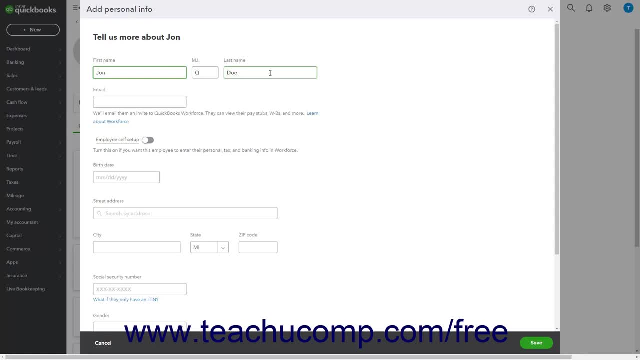 The email address that the employee has entered into the Payroll Setup field will appear in the Mail field. The address they used to view W2Info and PayStubs with QuickBooks Workforce appears in the Email field. The Employee Self-Setup toggle switch also appears below the Email. 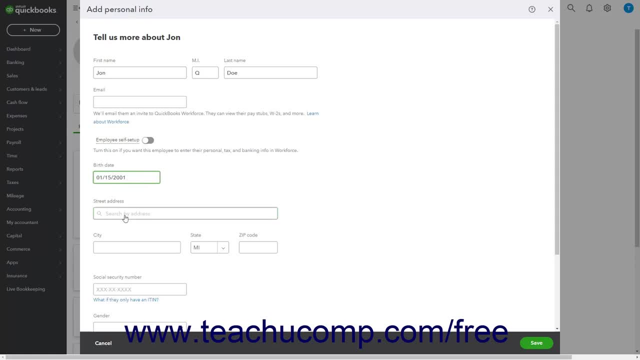 To enter their birthdate, type it into the Birthdate field. You can enter their address into the Street Address, City, State and Zip Code fields. Enter their Social Security number into the Social Security field. To enter their Social Security number, type it into the Social Security field. 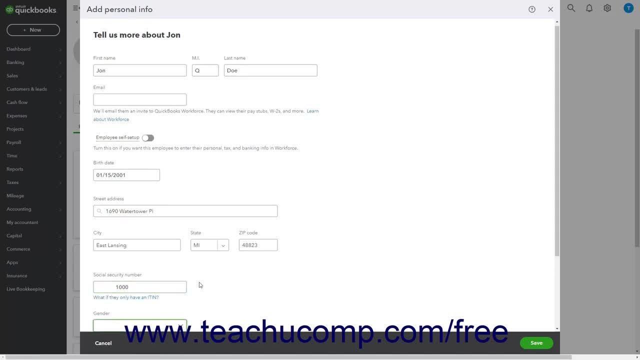 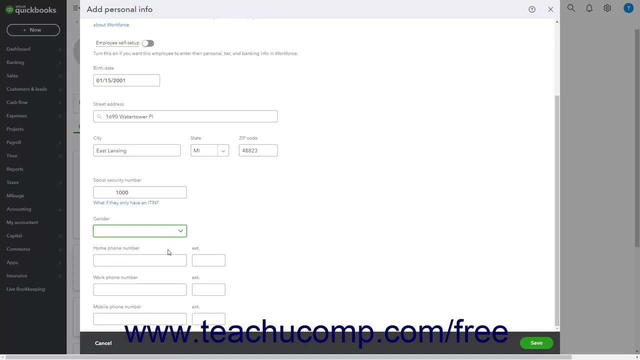 Social Security Number field. If needed to select a gender, select it. from the Gender field. You can enter contact numbers and extensions for their home phone number, work phone number and mobile phone number and associated extension fields. if needed To then save the personal information, click the Save button at the bottom of the Add Personal. 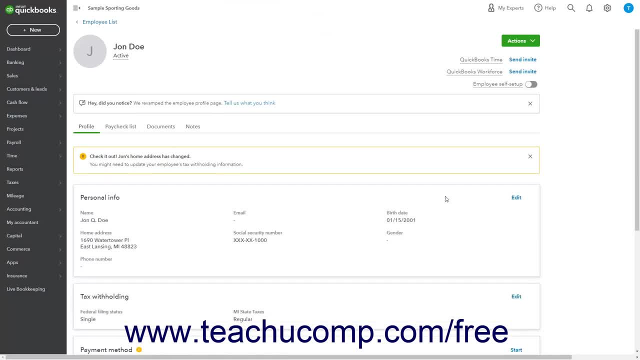 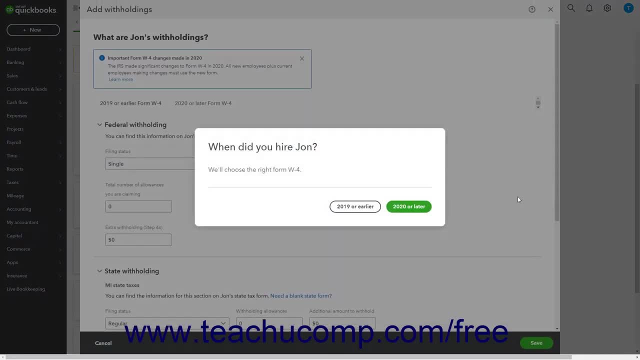 Info window. To edit the tax withholding information for the employee, click the Edit link in the upper right corner of the Tax Withholding section. Then click a button to answer when you hired the employee to select the correct W-4 form in the window that opens. 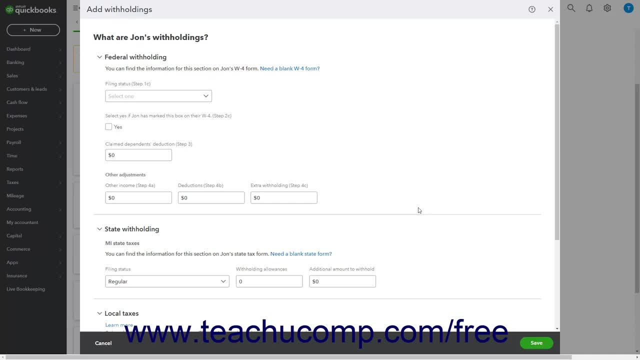 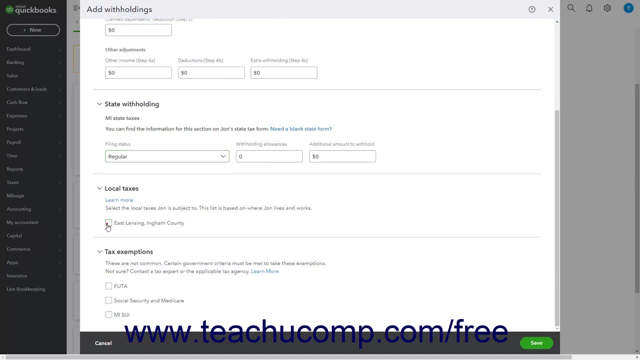 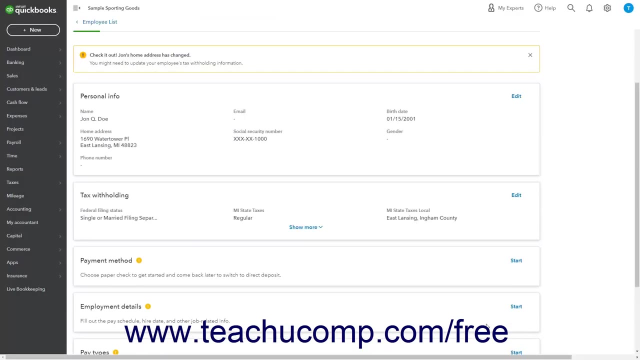 Then fill in the withholding information for the employee in the window that opens. After entering their withholding information, click the Save button at the bottom of the window to save it. To edit the employee's payment method, click the Start or Edit link in the upper right. 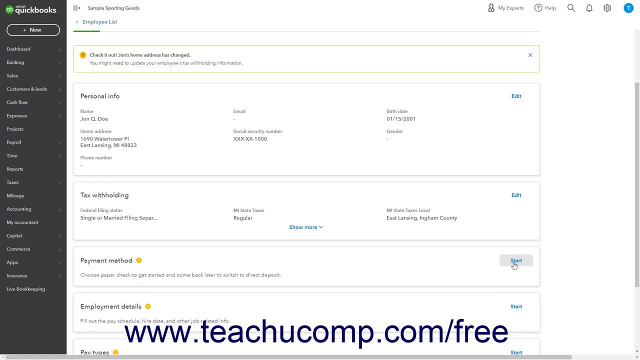 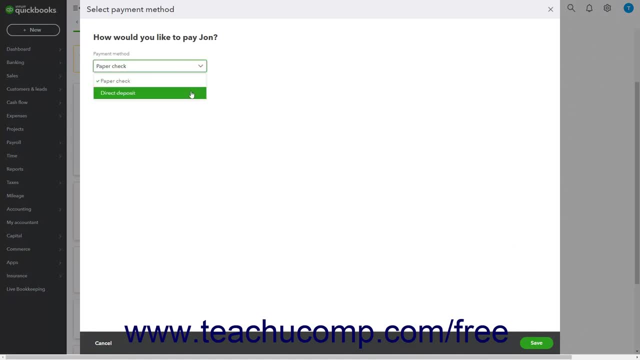 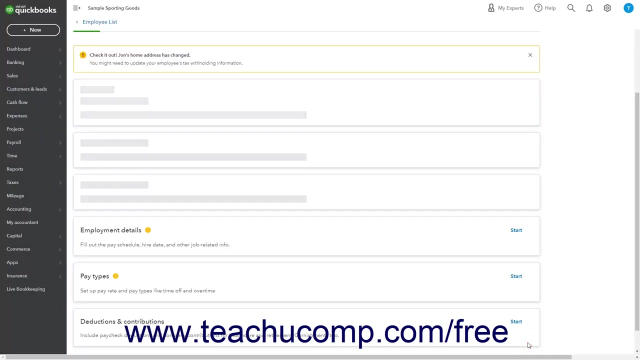 corner of the Payment Methods section to open a new window where you can select how to pay the employee from the drop-down For direct deposit. employees then enter their deposit method and enter the Related Banking information. To save this information, click Save. To enter the employment details of the employee, click the Start or Edit link in the upper right. 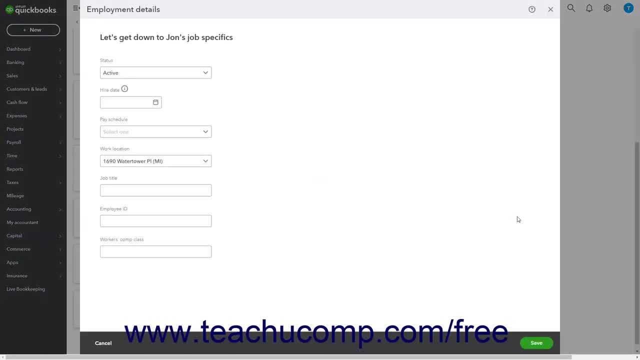 corner of the Employment Details section to open a new window. Select their employment status from the Status drop-down. Then enter the employee's hire date by using the Hire Date Calendar drop-down. Next select or create the pay schedule for the employee from the Pay Schedule drop-down. 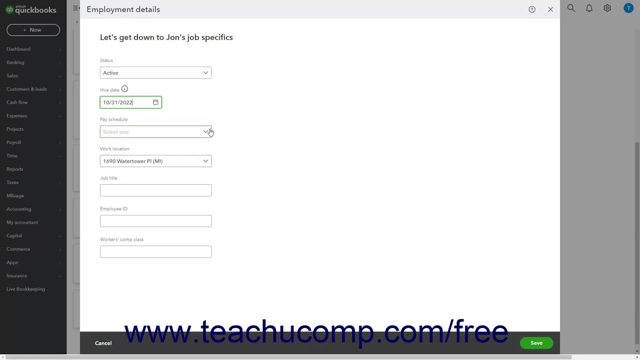 To enter the employee's hire date, click the Start or Edit link in the upper right corner of the Employment Details section to open a new window To enter the employment status of an employee, click the Start or Edit link in the Pay Schedule drop-down. 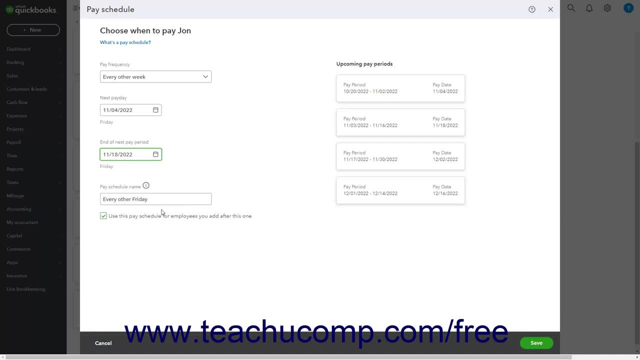 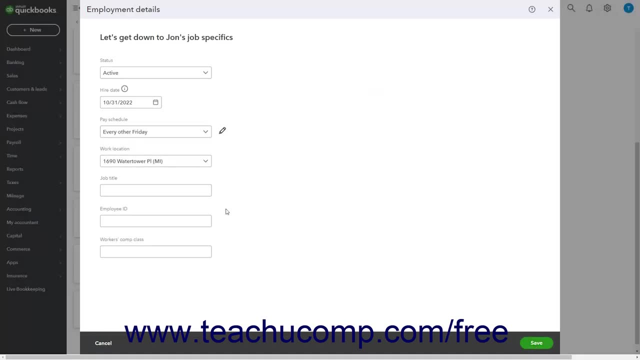 Next, select their work location from the Work Location drop-down. Select their work title from the Job Title Field and Employee ID from the Employee ID field. Once the title place entered into the Job Title field, click owners and floors automatically. The first year finger-picks areAccessed to the GAIS. first year holding: 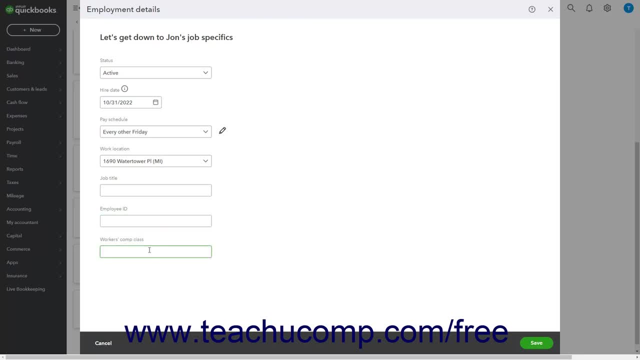 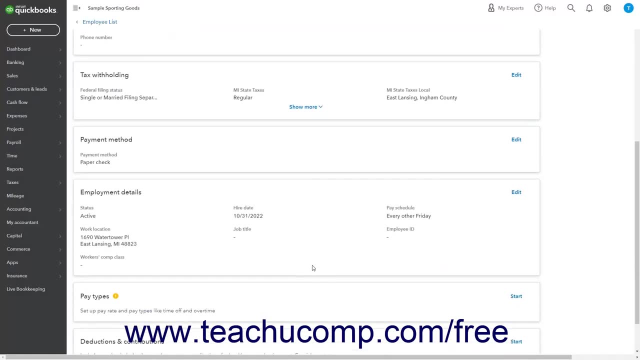 Then click Export To Uhm die action. Then click Order Worker's Comp Class into the Worker's Comp Class field. To then save the information, click the Save button at the bottom of the window To set the employee's wages and earnings. 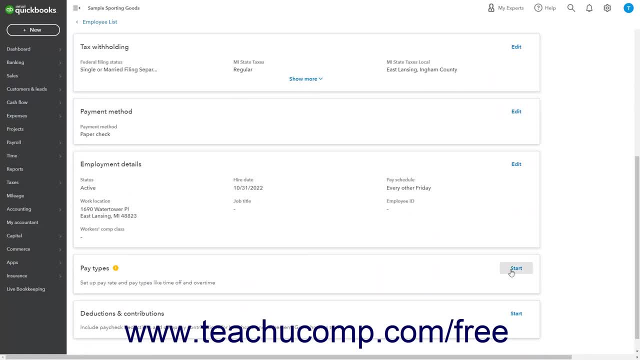 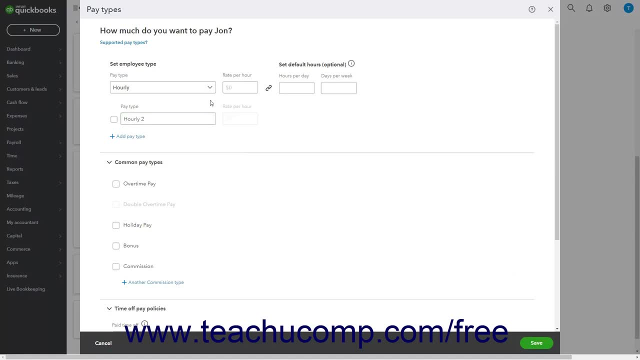 click the Start or Edit link in the upper right corner of the Pay Type section to open a new window. Then select the employee's type of wages from the Pay Type dropdown and enter the related hourly or salary information in the adjacent field or fields that appear Optionally for. 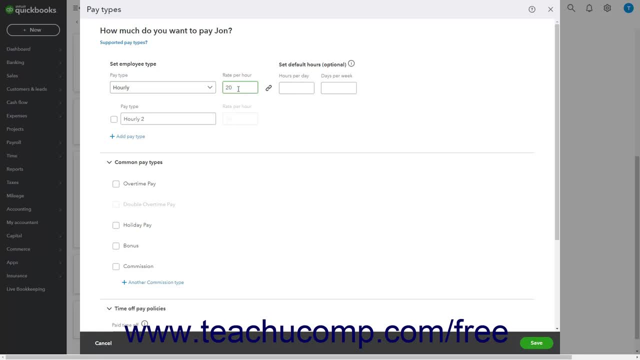 hourly and salary pay types also enter the default hours per day and days per week. they work in the next line of fields. To add additional pay types, click to expand the Additional Pay Types section if needed, and then check the checkboxes next to the 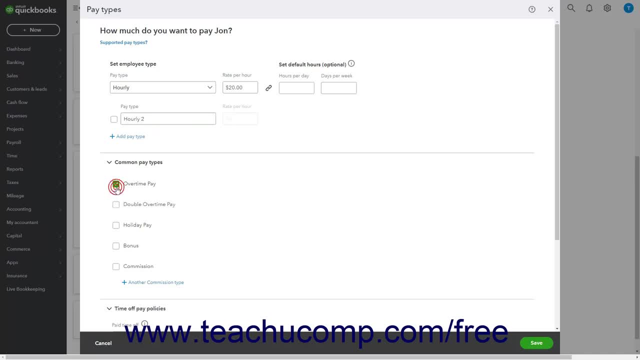 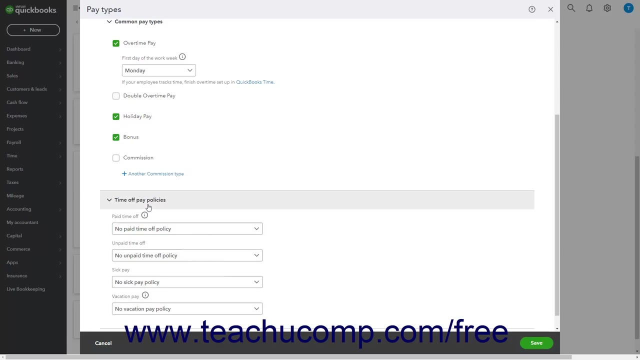 additional pay types to add. Then enter any information if needed for the selected pay types. To set time off pay policies, select a choice for each type of time off within the Time Off Pay Policy section. To save the pay type data, click the Save button at the bottom of the window. 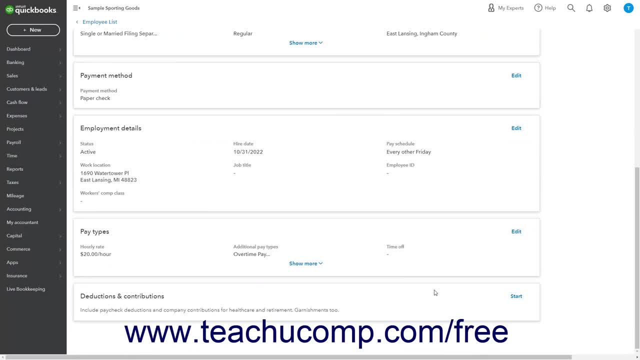 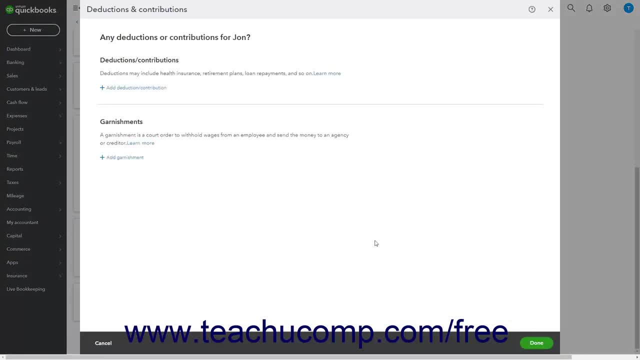 To enter deductions or contributions for the employee, click the Start or Edit link in the upper right corner of the Pay Types section to open a new window To then enter any deductions for the employee, like for retirement plans, garnishments or health care. click the Add Deduction, slash Contribution. 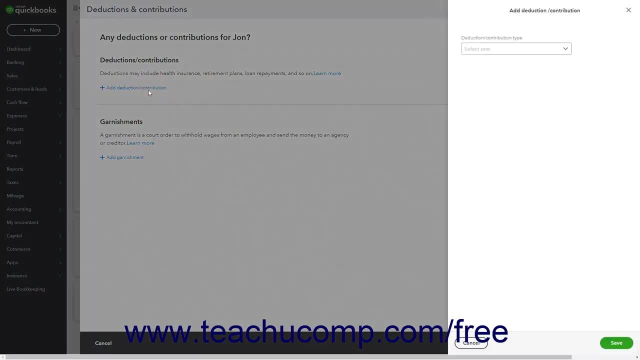 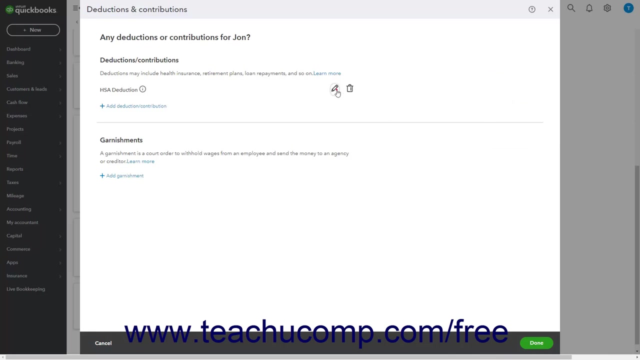 link to open a pane at the right side of the window where you can set up the deduction or contribution and then click the Save button at the bottom of the pane to save it If needed. you can then click the pencil icon for that deduction or contribution on this employee's page to edit its. 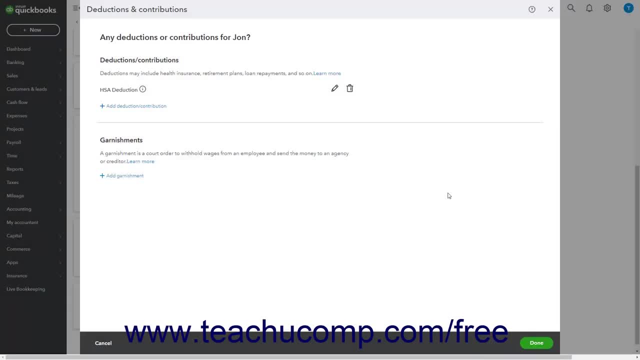 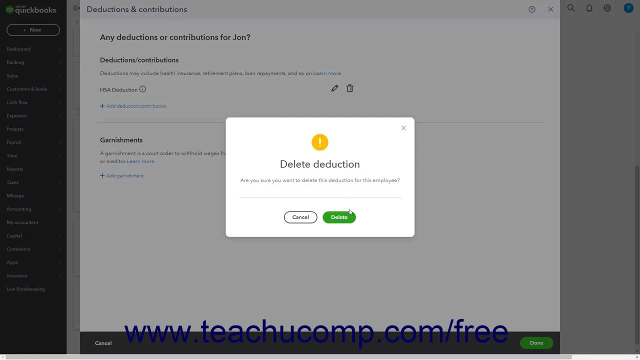 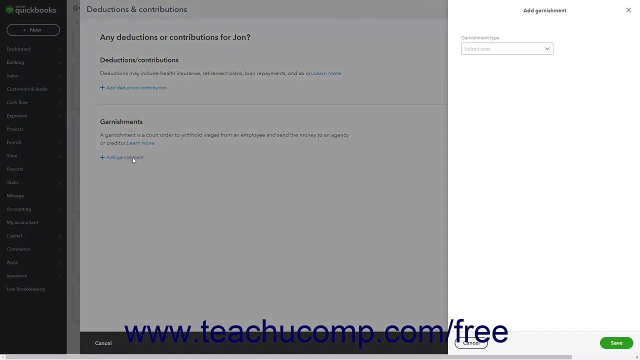 information for this employee. Alternatively, to delete the deduction for this employee, click the trash can icon and then confirm the deletion in the window that opens. To enter a garnishment for this employee, click the Add Garnishment link to open a pane at the right side of the window where you can set up the garnishment. 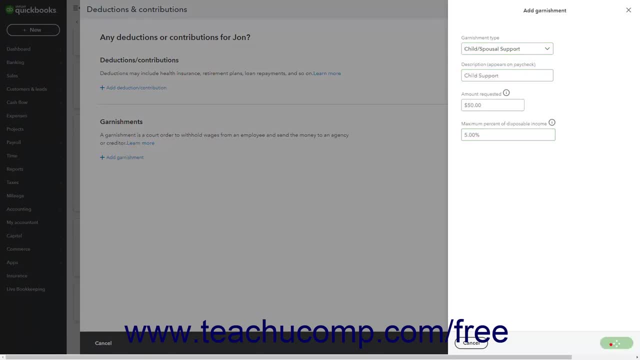 and then click the Save button at the bottom of the pane to save it If needed. you can then click the pencil icon for that garnishment on this employee's page to edit its information for this employee. Alternatively, to delete the garnishment for this employee. 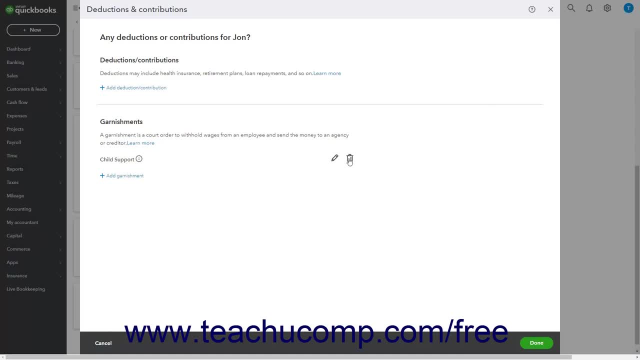 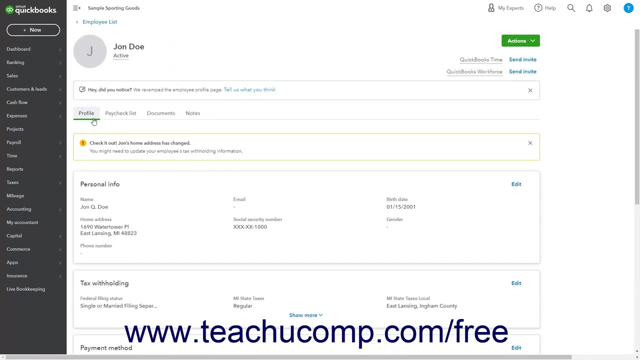 click the trash can icon and then confirm the deletion in the window that opens To close the deductions and contributions window. when finished, click the Done button in the lower right corner. In addition to the Employees Profile tab, there are also tabs you can click to show the employee's paycheck list. 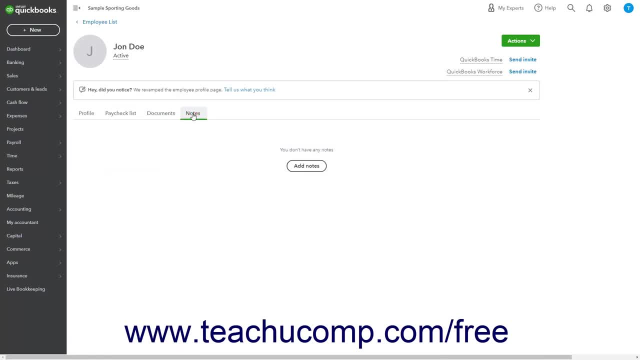 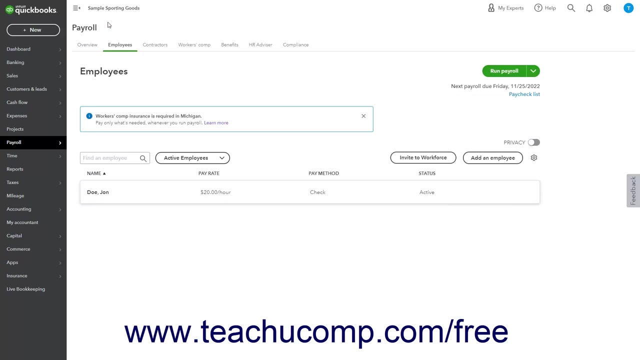 documents and notes. To return to the Employees list from an employee's page, click the Employee List link in the upper left corner of the employee page. After adding employees and running payroll, a graph showing your annual payroll cost appears at the top of the page. 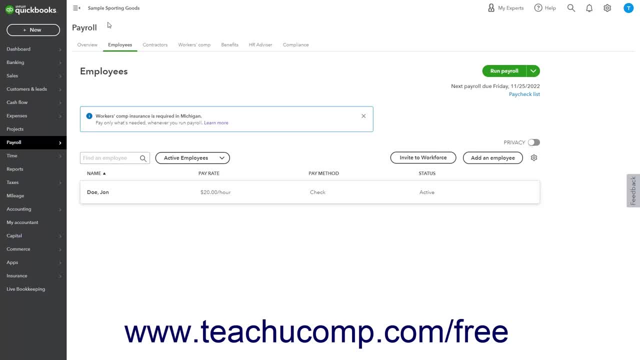 You can expand or collapse this section using the small arrow in the lower right corner of this section. Below this information is the Employees List. In the upper left corner is the Find an Employee field To find an employee in the Employees List. type their: 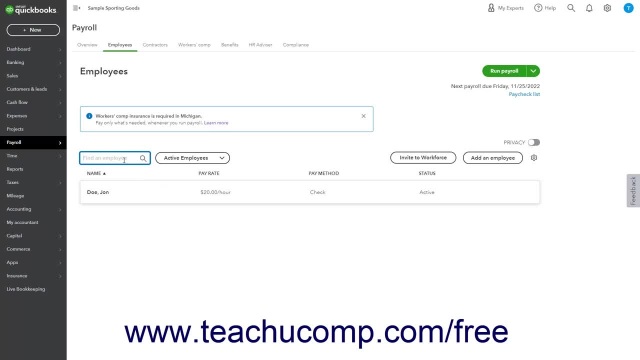 name into the Find an Employee field, which filters the list entries as you type. You can delete your entry from this field to show all employees again. The dropdown to the right of the Find an Employee field filters the Employees List to show active inactive.